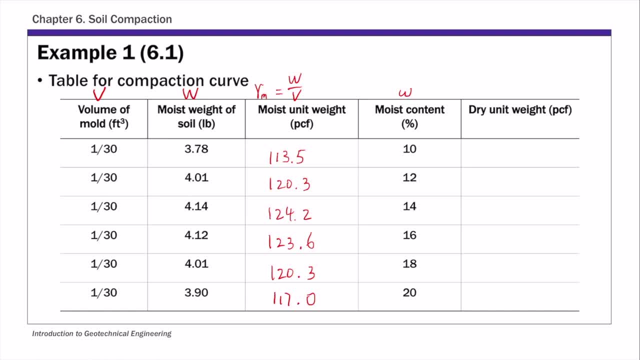 then we know the moisture content in percentage. So that's this fourth column. Then we can calculate the dry unit weight. Let's use gamma D for dry. So dry unit weight if you know the moist unit weight and if you know the moisture. 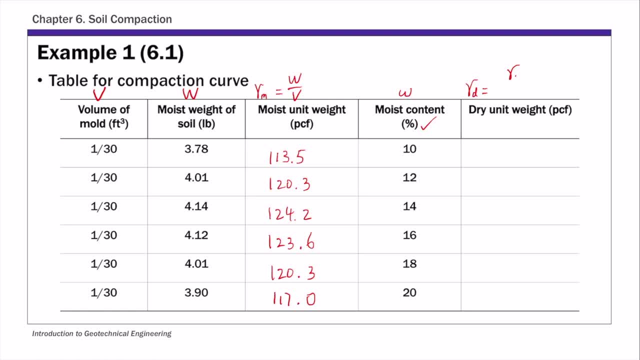 content. then gamma D is gamma M over 1 plus the moisture content, And since it's given in percentage, so we'll take that percentage number divided by 100.. So that's the dry unit weight. If you plug in those numbers from column 3 and column 4, then the dry unit. 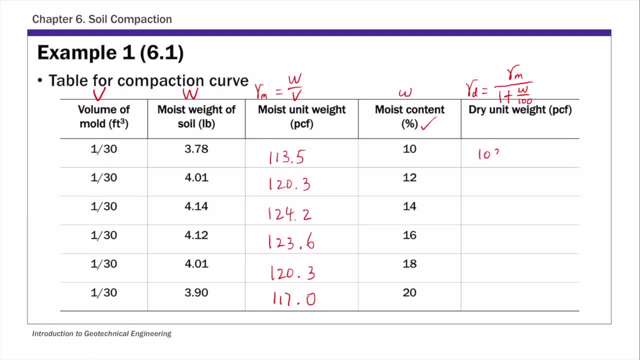 weight are 103.1,, 107.4,, 108.9,, 106.6,, 101.9, and 97.5.. Okay, So you have the dry unit weight here for this standard product to test, And then you can plot moisture content. So, basically, 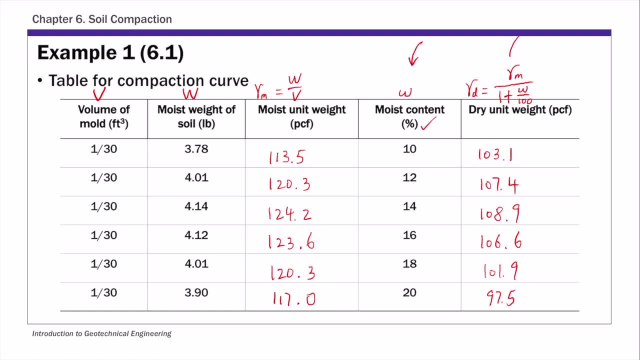 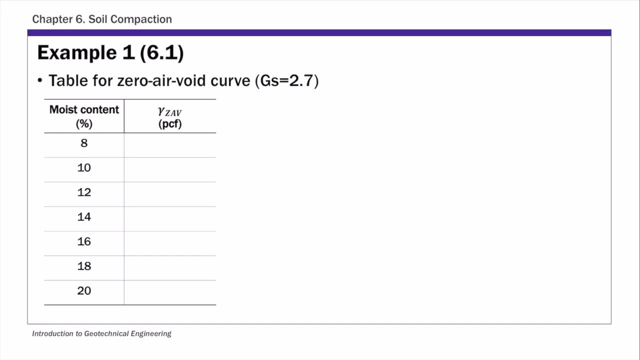 you can take moisture content column and the dry unit weight column and plot the compaction curve. And before we do that, so let's calculate the zero air void unit weight as well. So it's shown as gamma ZAV here, So let's plot this and let's calculate this and then plot it on the compaction. 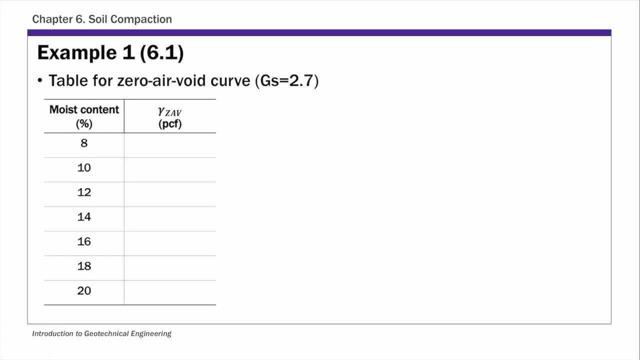 curve figure as well. So for gamma ZAV. so that's basically the dry unit weight corresponding to 100% degree of saturation, And we have derived that as in the previous lecture. So the expression for gamma ZAV is GS- gamma water over 1- plus GS W, which is the moisture content. 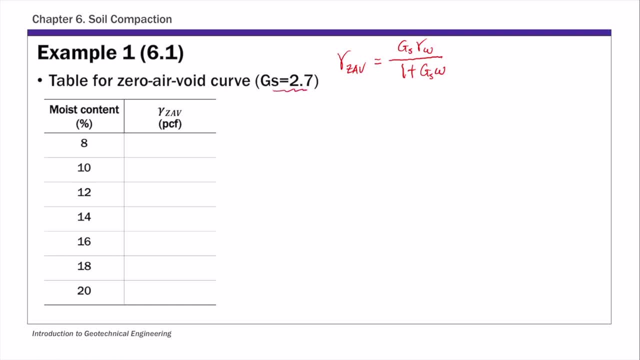 So then, if you substitute GS of 2.7 and moisture content as given in this column, So let's calculate the Gamma ZAV for moisture contents from 8% to 20%. A unit weight of water, gamma W is 62.4 pounds per cubic foot PCF. 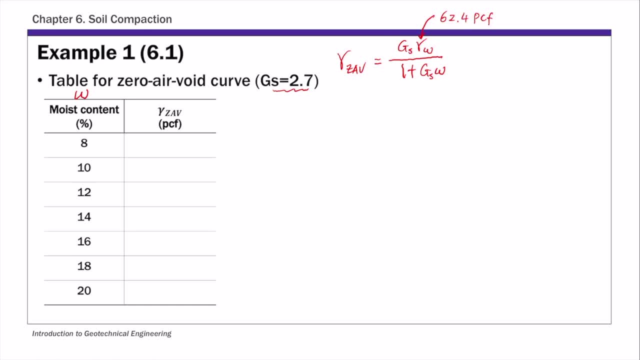 And if you plug in those numbers, then we have this column: gamma ZAV, as the first one is 138.6,, 132.7,, 127.3,, 122.3,, 117.7,, 113.4, and 109.4.. 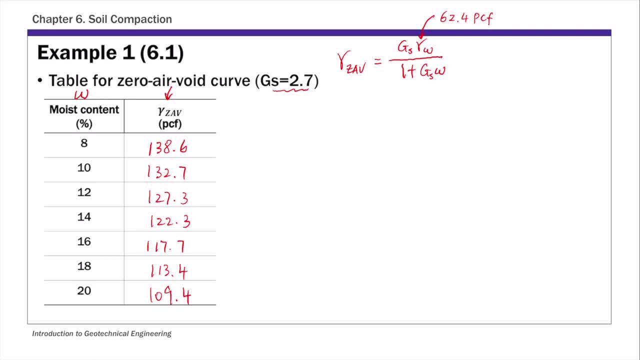 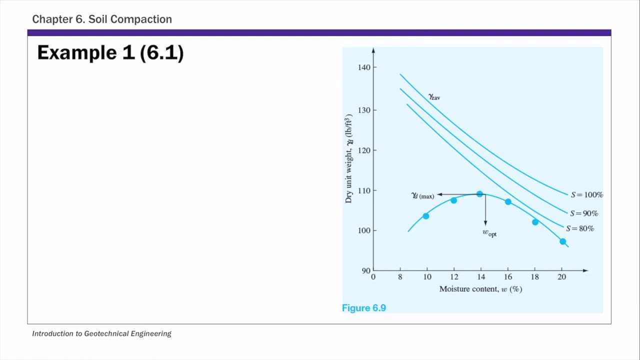 Okay, so we have another pair of data that we're going to plot on the compaction curve figure. So we have this omega or W moisture content versus gamma ZAV And this figure here shows there are- let's focus on just two curves on this figure. 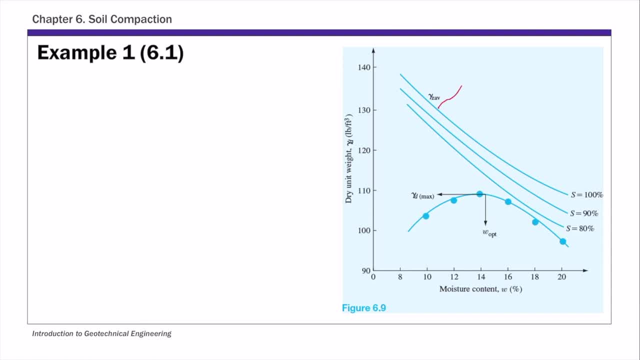 The first one is this: gamma ZAV curve. So this is gamma ZAV curve. So this curve, remember, by definition, that's the dry unit weight that corresponds to 100 degree, percent degree of saturation. So S is 100%, degree of saturation: 100%. 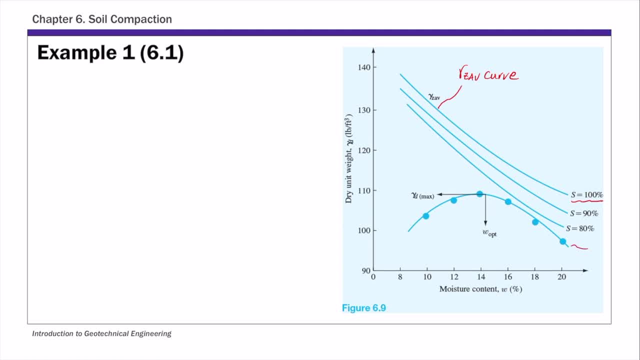 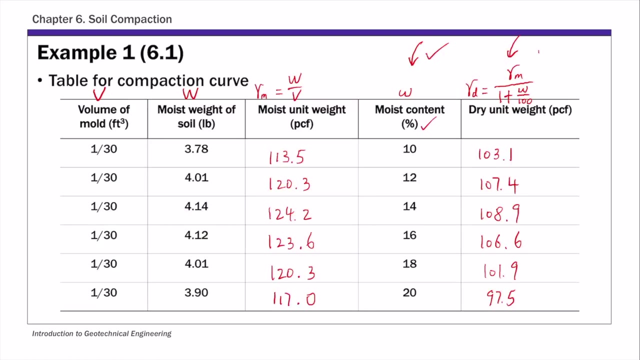 And then the second curve is this compaction curve here. So this curve, So all these dots, these are basically the moisture content versus the dry unit weight data. So that's this table here. So we're plotting this moisture content versus dry unit weight. 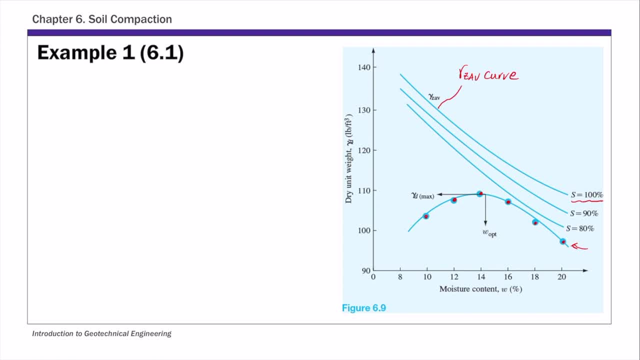 So these are the dots And then we connect those dots fit a curve that's a compaction curve, And from this compaction curve we can get the dry maximum dry unit weight. So that's a unit weight based at the top, the peak of this curve. 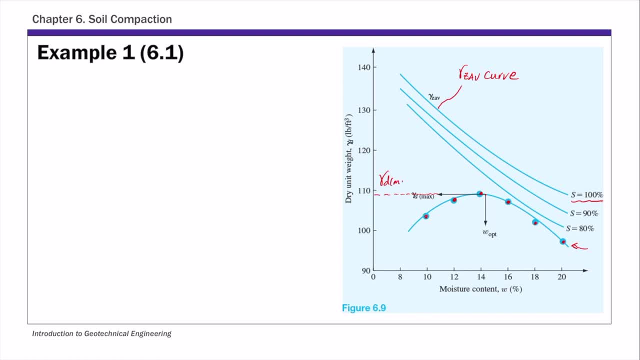 So that gamma D max is what we are looking for, And for this example it's about 109 pound per cubic foot PCF And then the corresponding X value, So that's a moisture content corresponding to gamma D max. So that's called the optimum moisture content WPT. 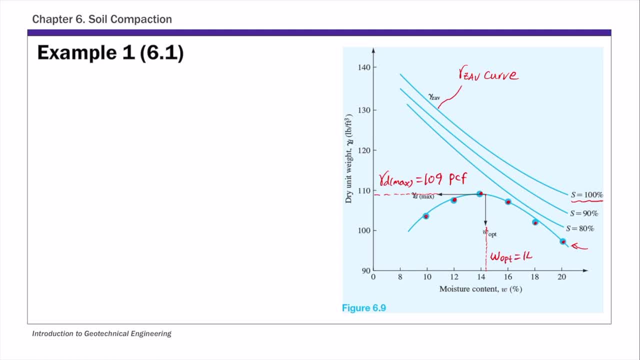 And it's approximately 14.4%. So that's the example one, And we plotted both the compaction curve and gamma ZIV And notice that its compaction curve lies to the left of gamma ZIV as expected. And then this peak point on this compaction curve.